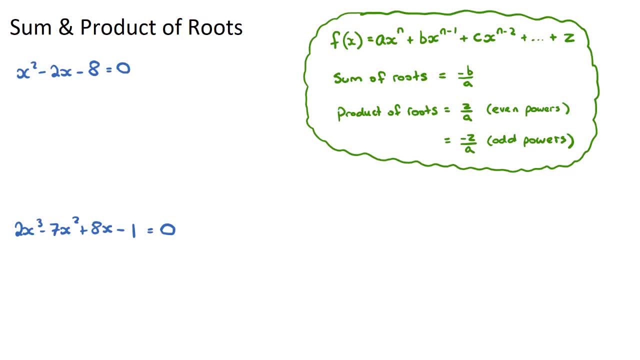 In this video we're going to have a look at the sum and product of roots of a quadratic and any other polynomial equation, So we need to understand what this formula is telling us and how to apply it to some common IB maths exam questions. Okay, so if I have a quadratic equation like I have here, x squared- 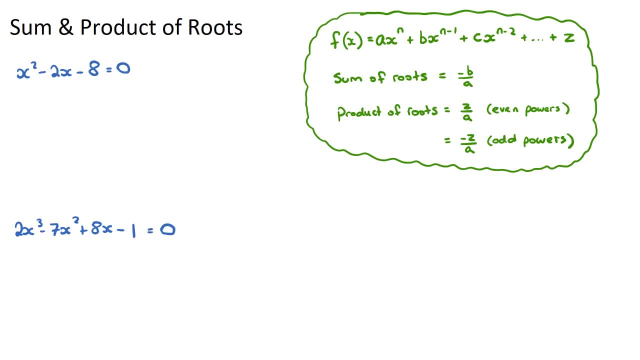 minus 2x minus 8, we know this has two roots, and roots are when this equation, if we were to graph it, and this would look a little bit like this here, where the roots would actually be at negative 2 and 4.. We could find that if 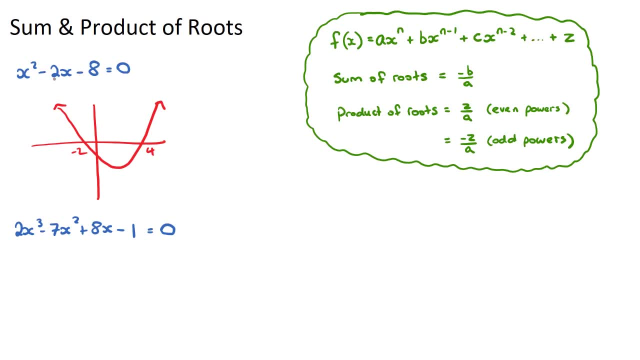 we factorized it and did the null factor law, or if we graphed it on our calculator. but the sum of the roots is just summing up the two values of our roots of this equation. So that's what the sum of roots means and the product. 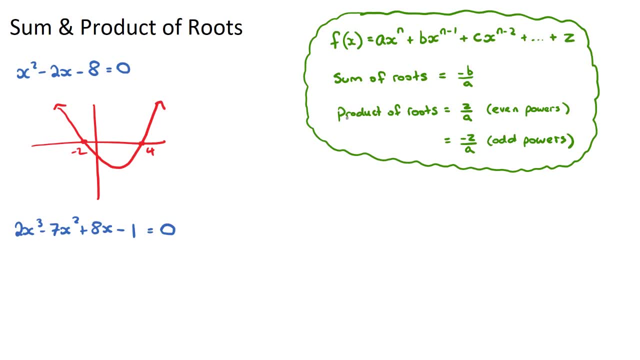 is just the multiplication of these two roots. So this is a very important topic when we look at some higher order polynomials And also some complex numbers. Okay, so the sum of roots formula says that the sum of the roots of any polynomial will be negative. b on a, which is a, is the 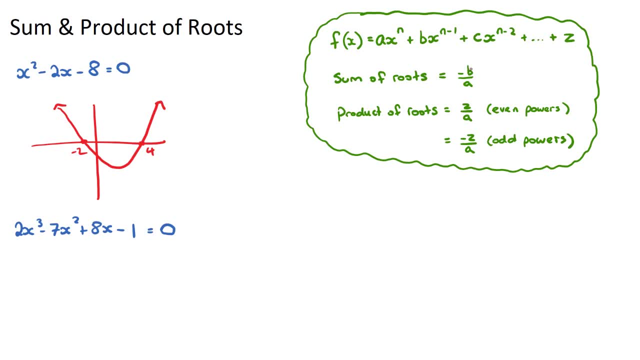 coefficient of our largest power and b is the coefficient of the the next term. It's the term with one less in the power here. So it's very important that if x to the power of 7 is our largest power, b is the coefficient of x to the power of 6.. 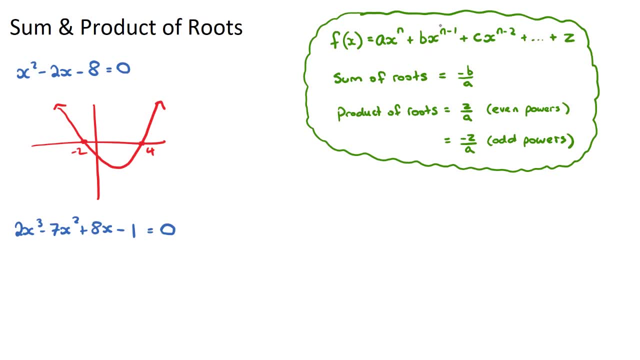 It's the one one below it. Now, if there's no coefficient to x, to the power of 6, if there's no term, the coefficient is actually 0. So we will look into that. Okay, so with our quadratic here, if we apply the sum of roots, sum of roots, the equation says: 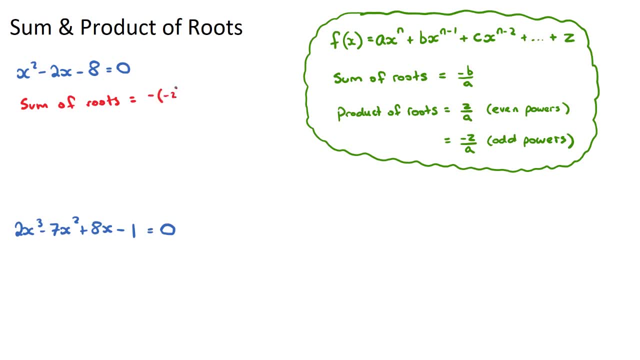 it'll be negative b, so it'll be negative negative 2 over 1, which will just be 2.. Which is accurate to our drawing before, because our two roots were negative 2 and 4. And if we were to sum these, we would get positive 2.. Now, the product of our 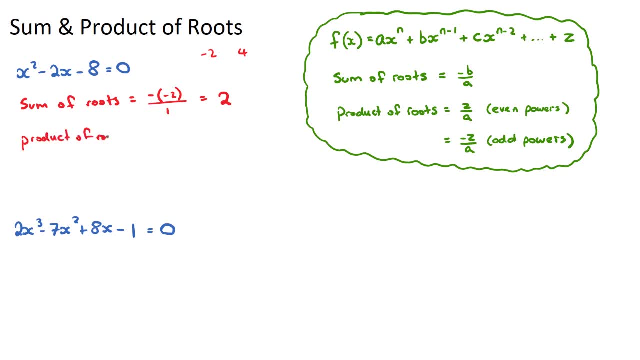 roots, product of roots, the product of roots formula. the answer is z on a, So it's the constant term over the coefficient of our largest term. And it's positive z on a if our polynomial has an even power, So a quadratic x to the power.